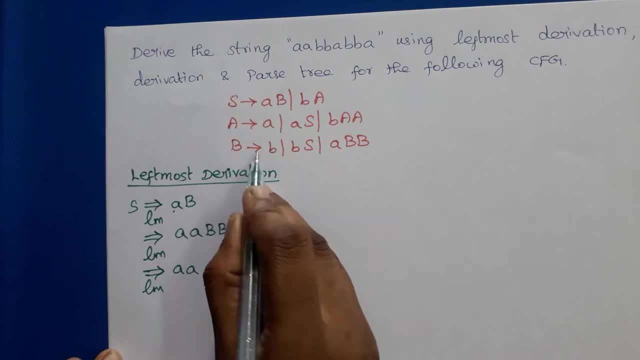 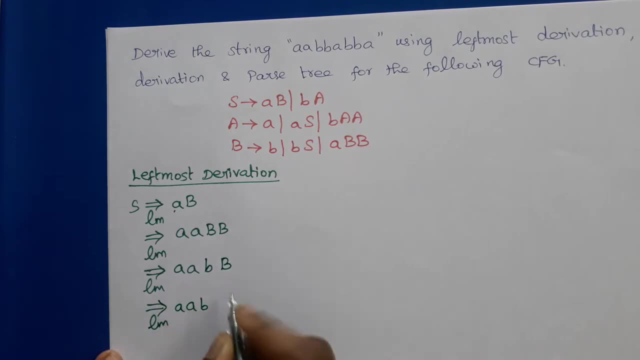 So we can use this production. So B tends to B, So B can be replaced by B. Now the leftmost non-terminal or leftmost variable is B. Fourth symbol is B. So we cannot use this And we may not apply B also, because if you substitute B here, then we cannot derive. 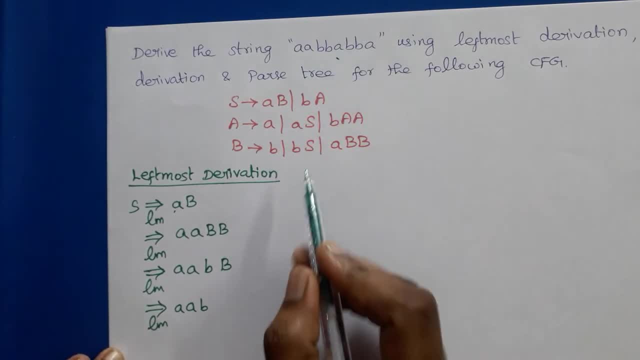 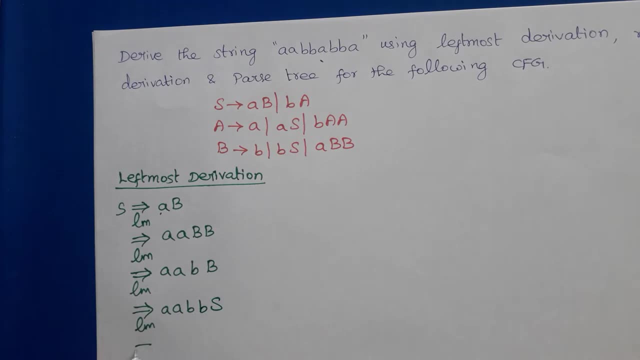 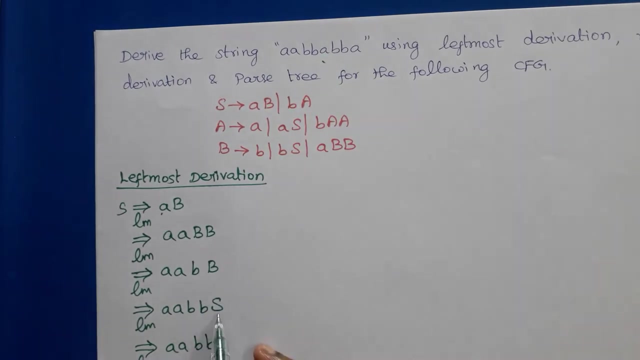 the rest of the input symbols in the input string. So we have to use BS, So B must be replaced by BS, Then AABB, So next we need A, So S is the leftmost variable, So S must be replaced by AB. 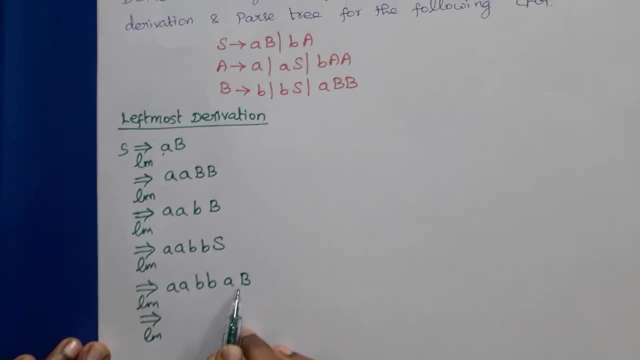 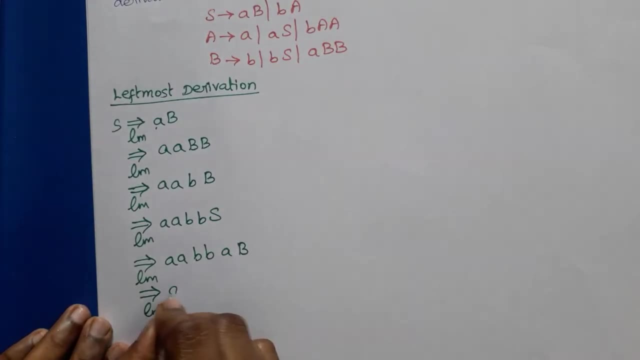 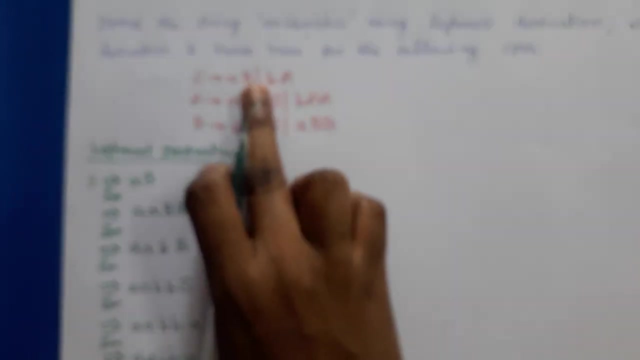 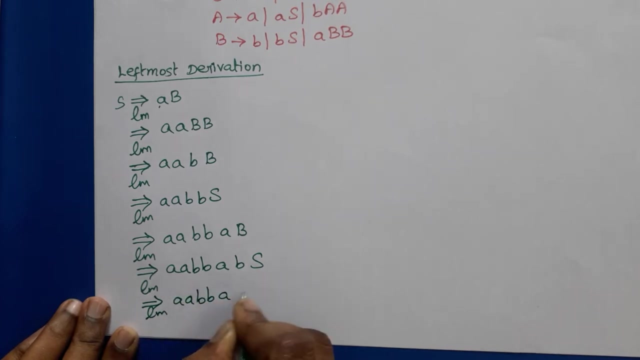 Next, the leftmost variable is B, And we need B here. So B must be replaced by BS. AABBABS: Again: we need B, So this S must be replaced by BA. Again, we need B, So S must be replaced by BS. 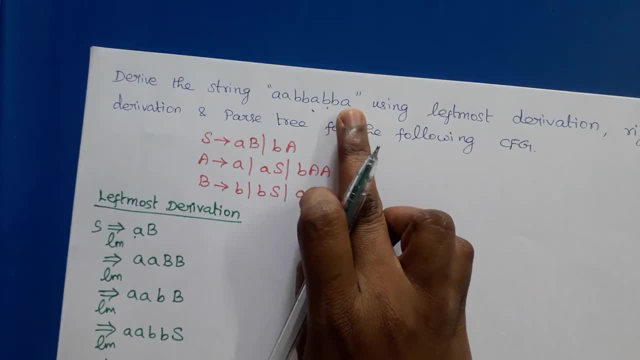 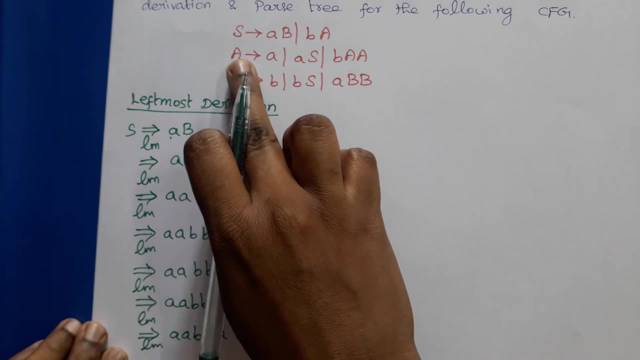 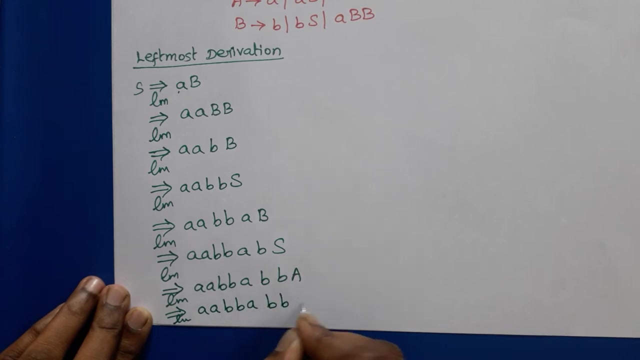 and now we need a yay, yay in there, a as a loss symbol. So chase this leave. the A is the leftmost variable, So this must be replaced by a BBAununth. So we have derived this train from the start symbol of the grammar using leftmost variable, so 위에. 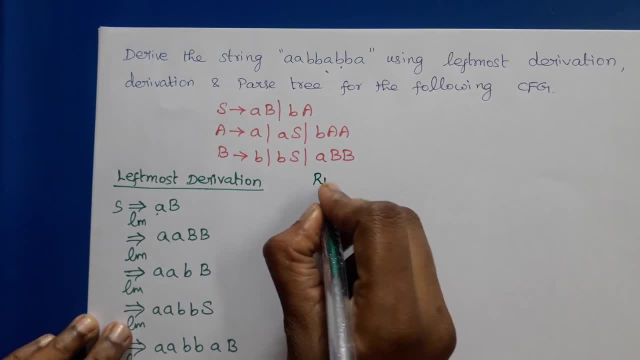 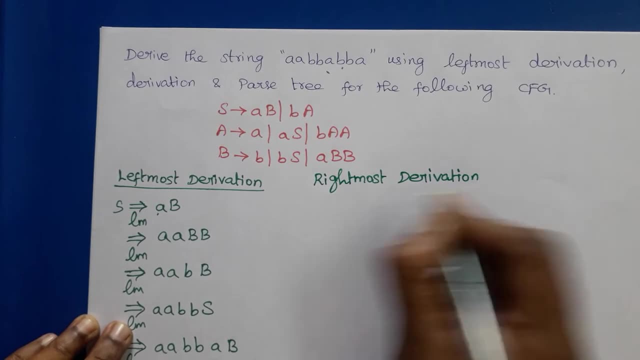 And BBA. So we need A as the last symbol. So this variable, A, is the leftmost variable, So this must be replaced by A leftmost derivation. Now we will construct the rightmost derivation, So we need to start. 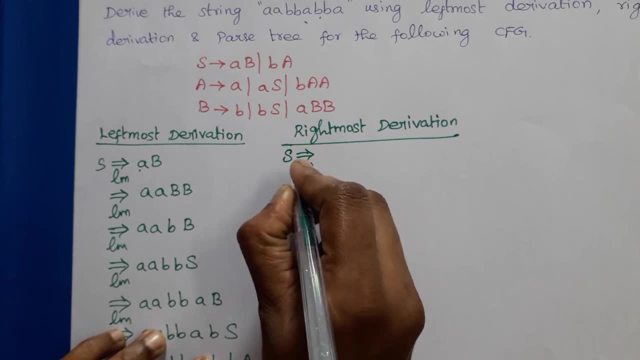 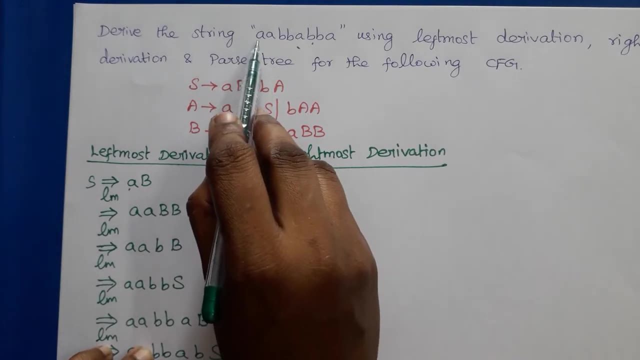 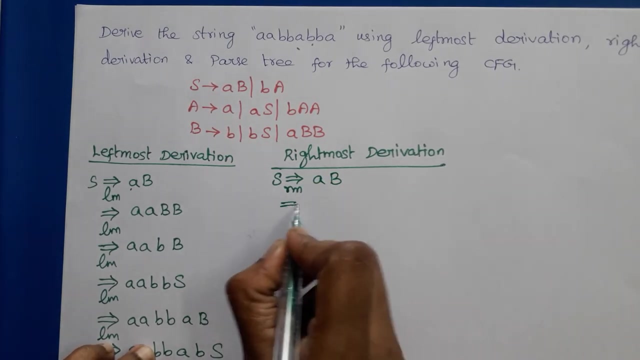 with the start symbol of the grammar. So yes, in rightmost derivation. Here the rightmost variable is yes, So it can be replaced by any one of the production body. Again, we need a, So we have to replace yes, derives a, b. Then the rightmost non-terminal symbol is: 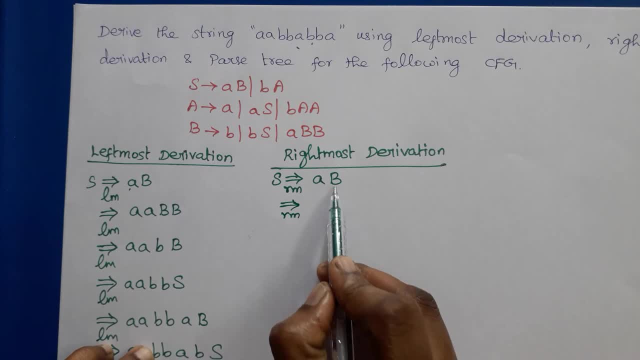 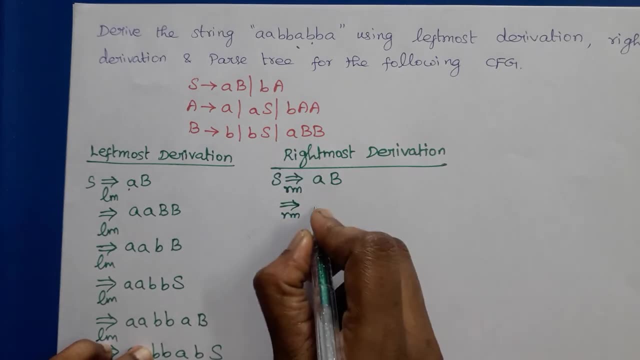 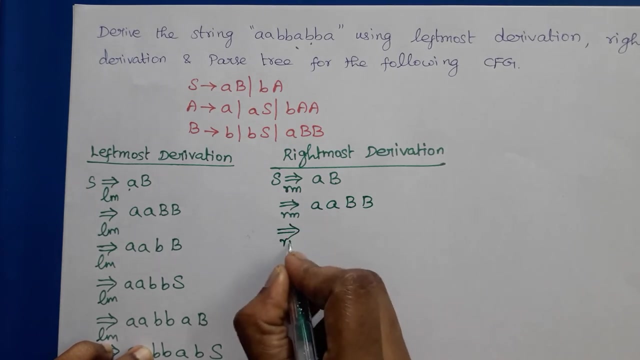 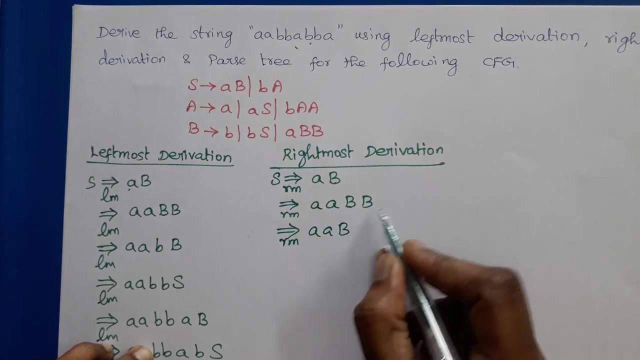 b, So b. So here b can be replaced by any one of the productions, So we may take this: a b, b, So b is derived as a b b. Now, in this step the rightmost non-terminal symbol is b, So we need to write the remaining symbols as it is And b b can be replaced by b is. 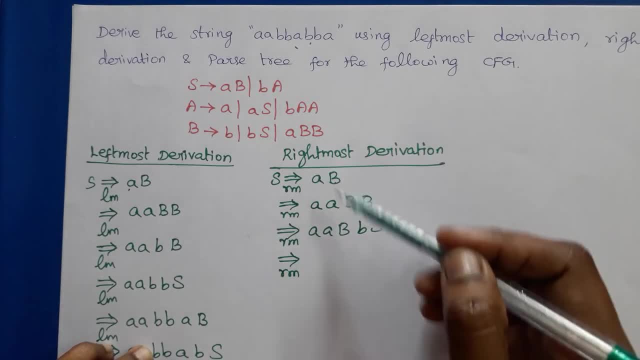 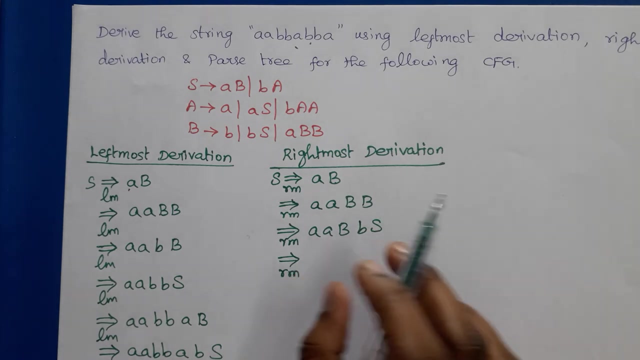 If you can't get, you can't derive the string properly, for by applying the wrong production we can do it again with the. we have to backtrack it and do it again. So in the rightmost derivation we cannot predict the exact production at each step. 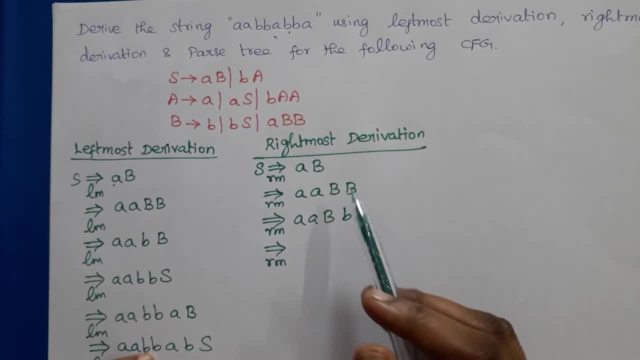 But we can do it again with the. we have to backtrack it and do it again. So in the rightmost derivation we cannot predict the exact production at each step. So here b, b or b is derived as a, But if the string is correct string, definitely we can construct the rightmost derivation. 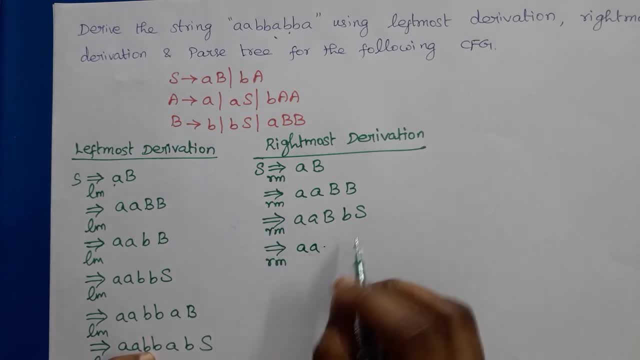 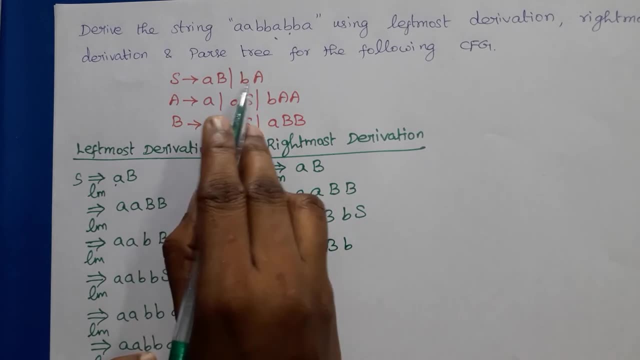 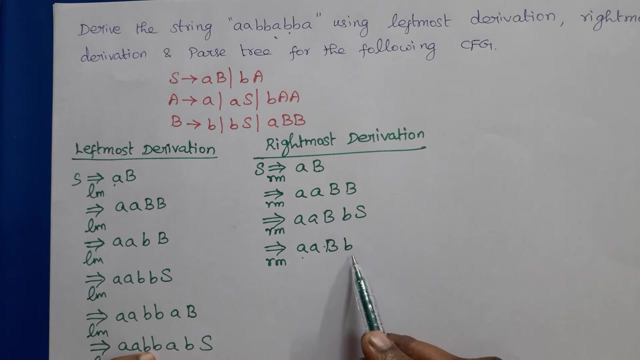 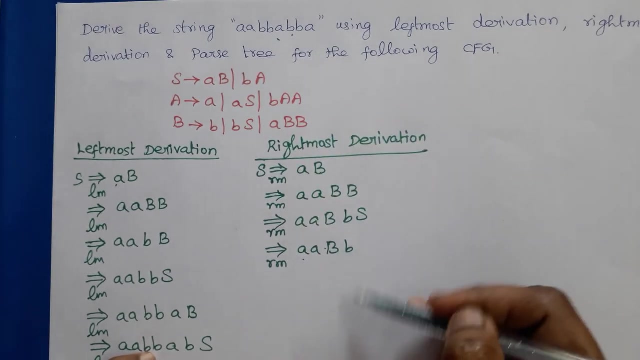 also for the same string. So a, a, b. In this step the rightmost symbol is yes, So yes must be replaced by in any one of the production body. Here, see, we have got a a and one non-terminal symbol is there. Again, we have got one b, So we need to try to retrieve another, this b a, here. So you. 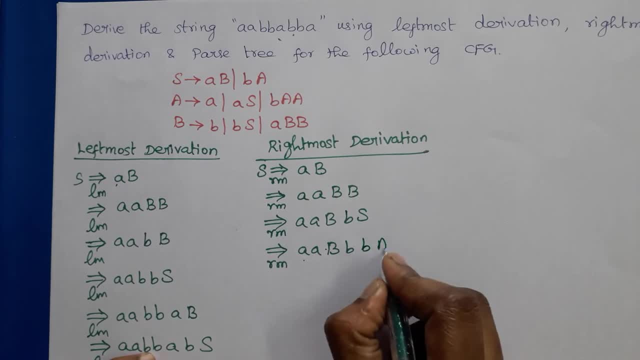 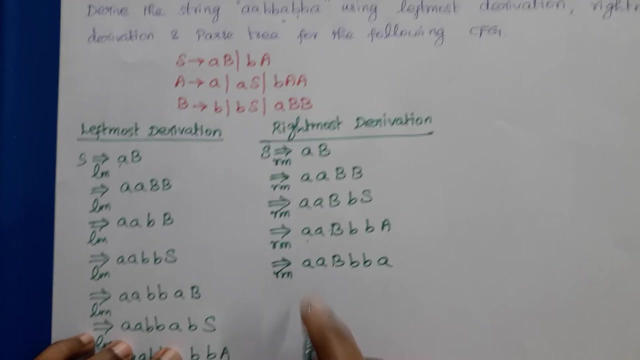 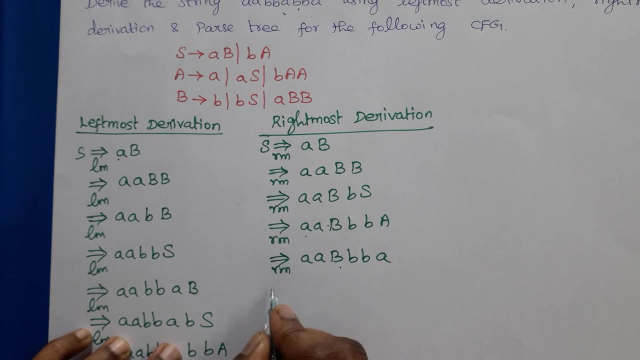 yes, must be replaced by ba, right ba, and this a a is a rightmost variable. this a can be replaced by a, the first production. so a, a, b, b, b a. now we have got first two symbols in the last b, b a. so now we need to retrieve b, b a from this b. so 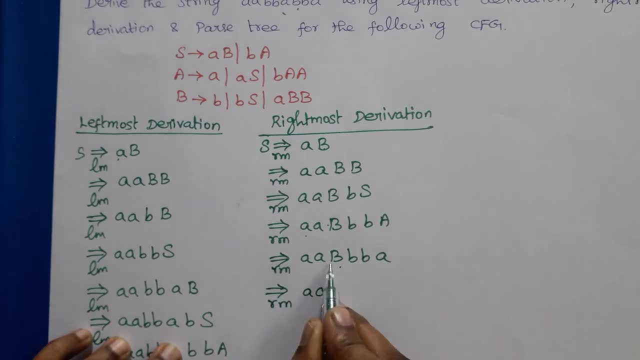 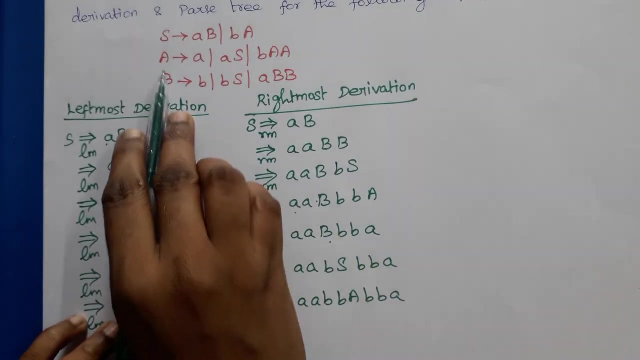 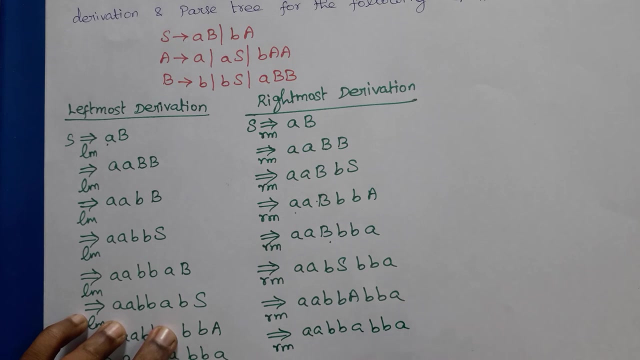 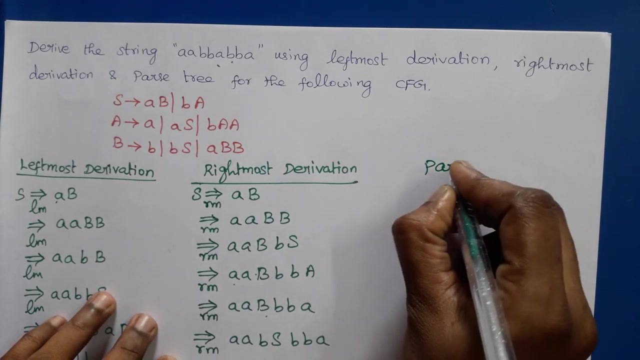 the rightmost variable is b, and b must be replaced by bs. then, in the next step, the rightmost variable is s, s must be replaced by ba, and, and now we need a a, so a should be replaced by small letter e. so so we have derived a a, b, b a, b, b, a from yes, using rightmost derivation. next we need to: 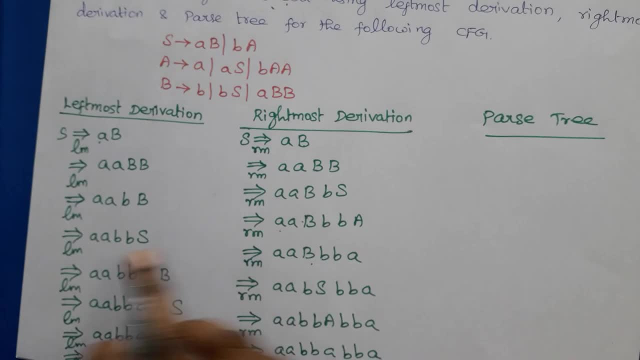 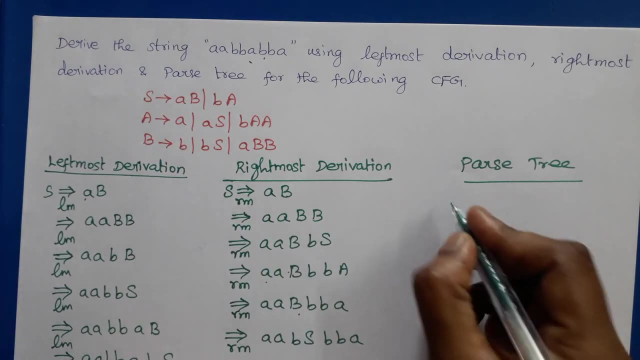 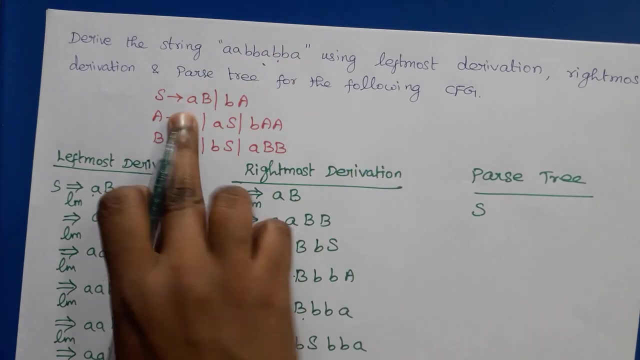 construct a parse tree. so to construct the parse tree, we can either follow the leftmost or rightmost derivation or simply you can derive the string from the grammar directly. so yes, is the root of the parse tree. we can use either this or this, but we need this input string, so the suitable one is: